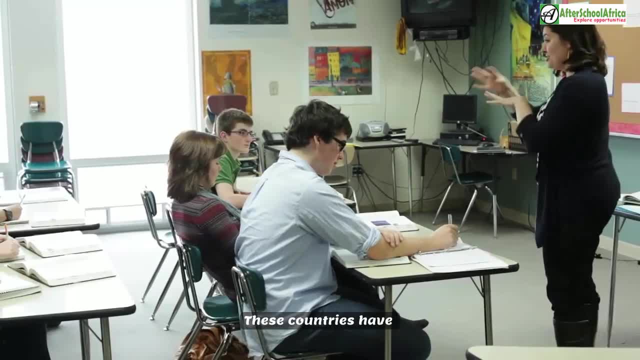 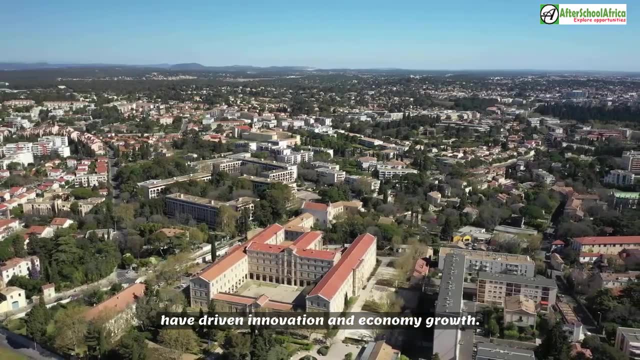 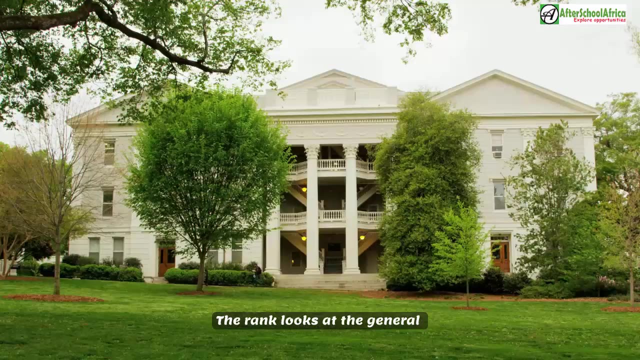 countries can learn from them. These countries have developed unique, world-class education systems that have driven innovation and economic growth. This ranking is according to the Global Competitiveness Report by the World Economic Forum. The rank looks at the general level of skills of the workforce and the quantity and quality. 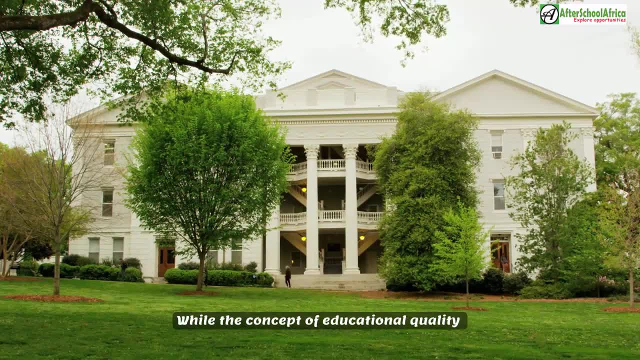 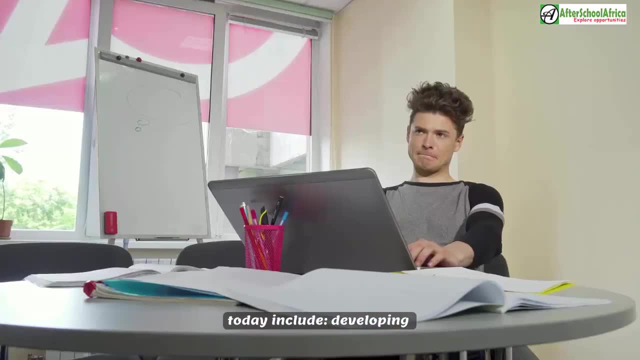 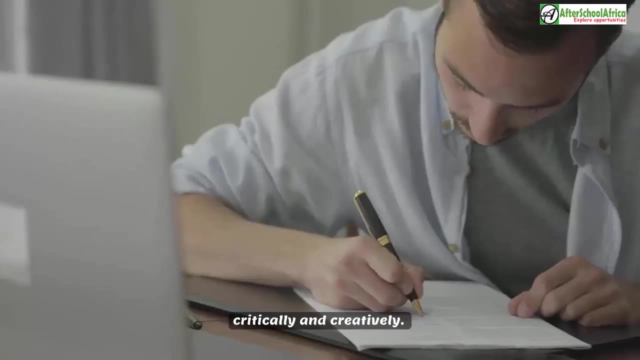 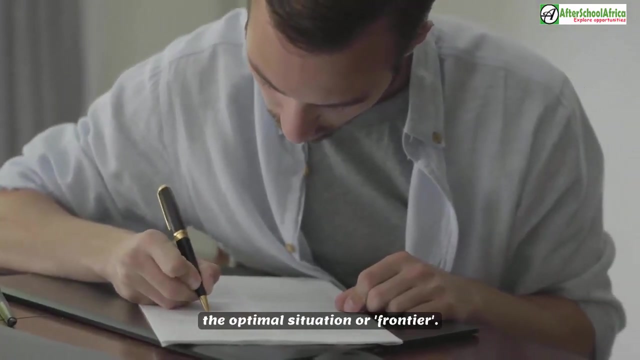 of education in each country. While the concept of educational quality is constantly evolving, important quality factors today include developing digital literacy, interpersonal skills and the ability to think critically and creatively. Scores are on a 0 to 100 scale, where 100 represents the optimal situation or frontier. Canada and Australia tied up at 11.5.. The United Kingdom followed at 13th position with 81 points each. The United Kingdom followed at 13th position with 80.2 points. So which countries are the top 10?? 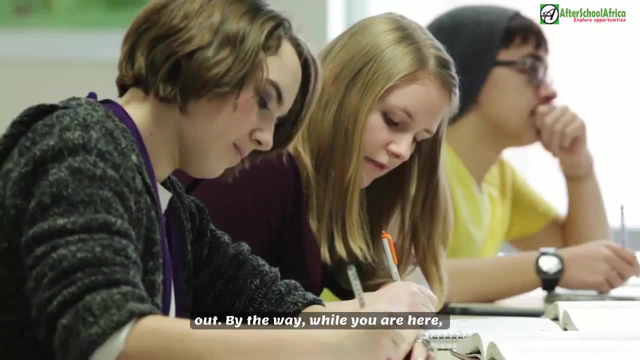 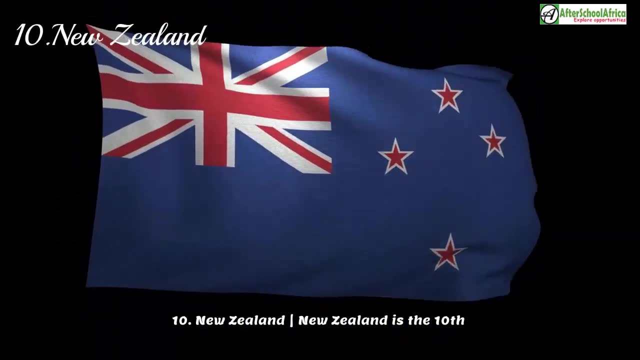 You ask, Let's find out. By the way, while you're here, consider subscribing to After School Africa for more educational videos like this. 10. New Zealand: New Zealand is the 10th country with the best education system in the world. 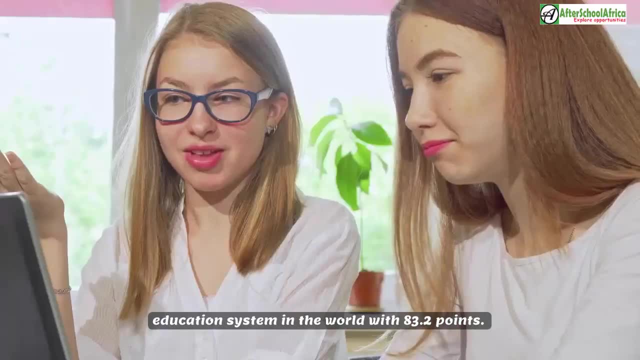 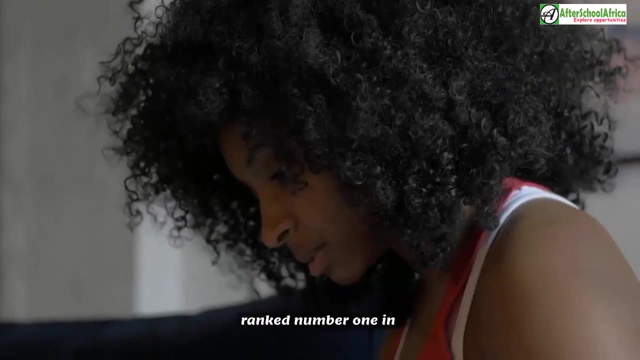 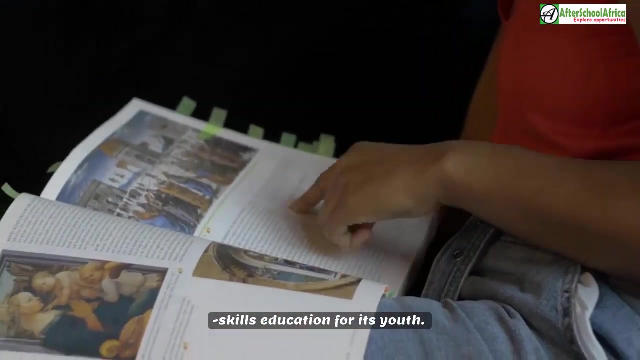 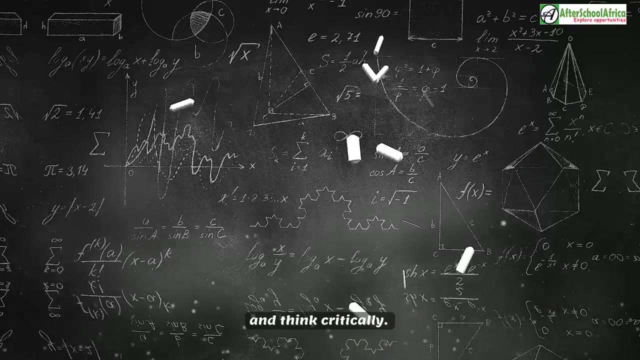 With 83.2 points, It ranks 5th position for critical thinking in teaching. The country is also ranked number 1 in the world by the Economist Intelligence Unit for providing future skills education for its youth. The education system encourages students to ask questions and think critically. 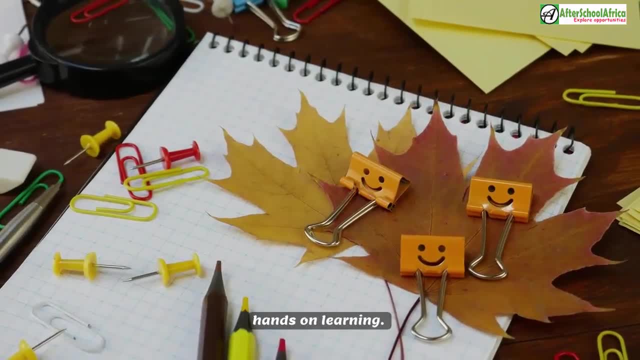 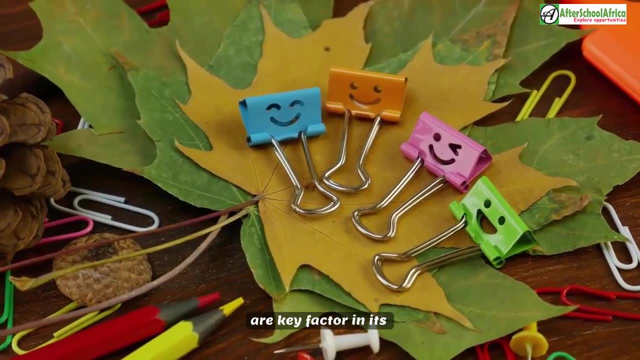 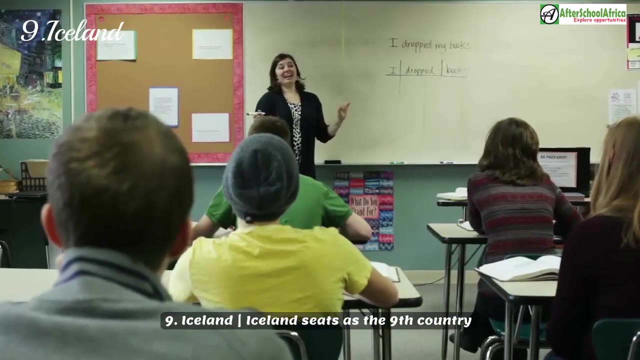 Teaching styles offer practical and hands-on learning. The quality of teaching And an underlying culture focused on children's learning are key factor in its successful education system. 9. Iceland. Iceland sits as the 9th country with the best education system in the world. 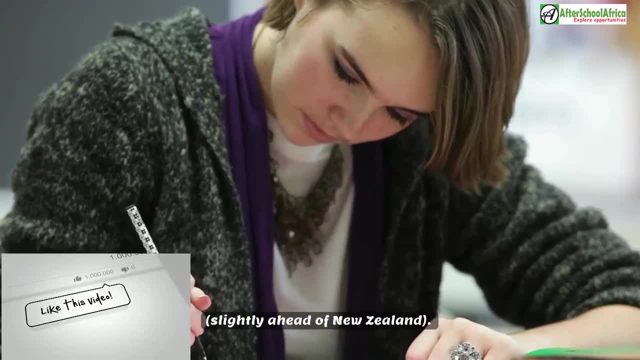 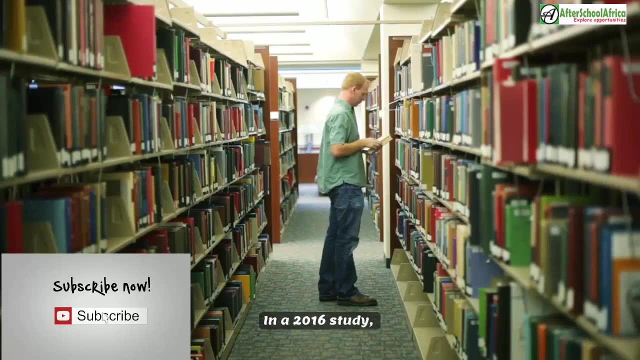 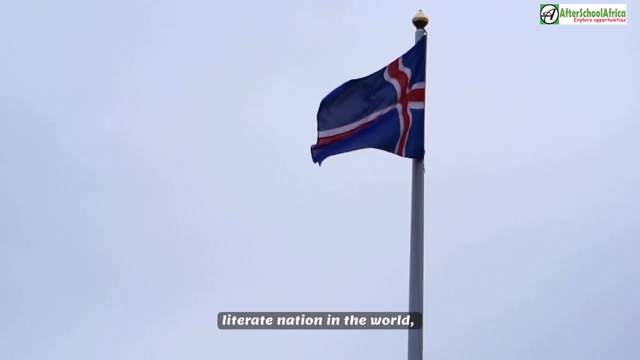 With 83.3 points Slightly ahead of New Zealand, the country ranks 4th position in school life expectancy. In a 2016 study, Iceland was ranked the 3rd most literate nation in the world, trailing behind Finland and. 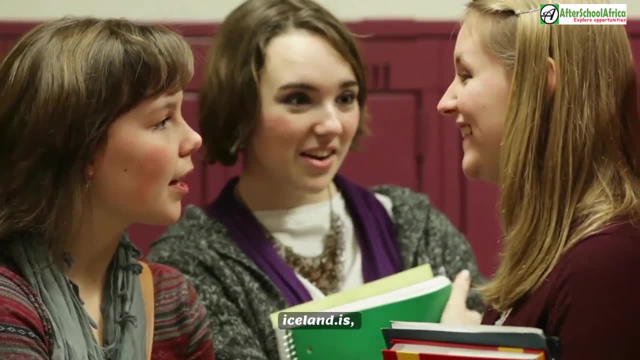 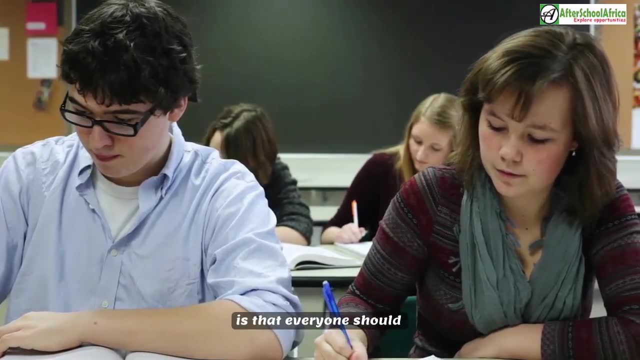 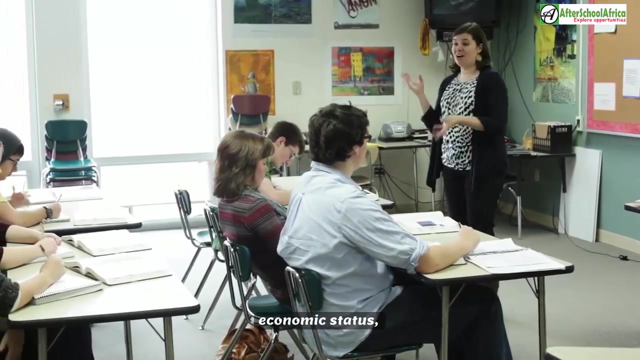 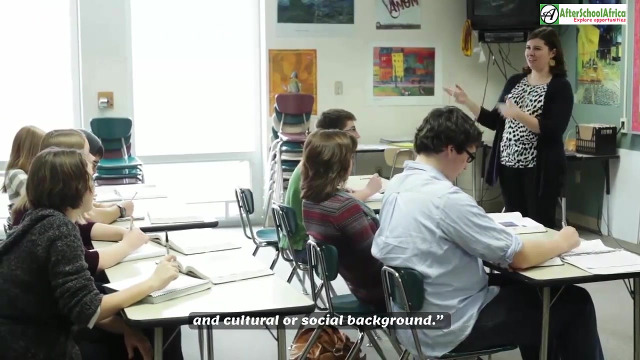 Norway. According to the nation's website, Iceland is. a fundamental principle of the Icelandic educational system is that everyone should have equal opportunities to acquire an education, irrespective of sex, economic status, residential location, religion, possible handicap and cultural or social background. 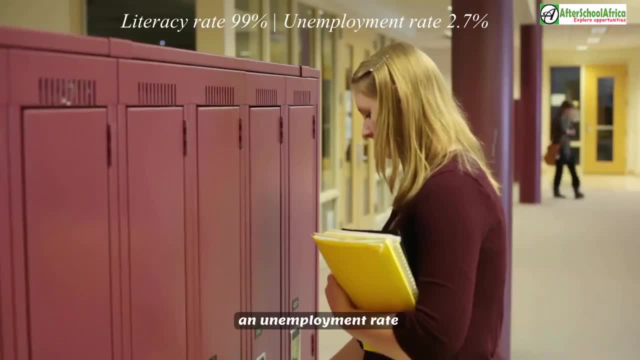 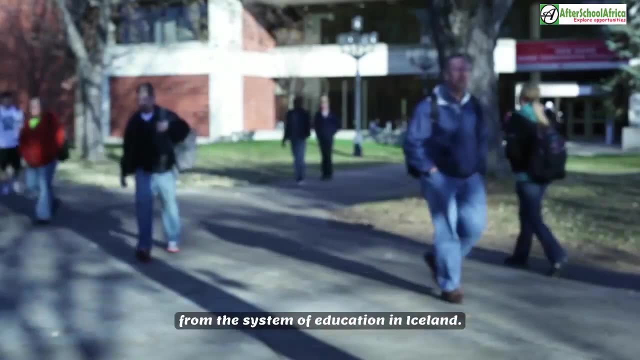 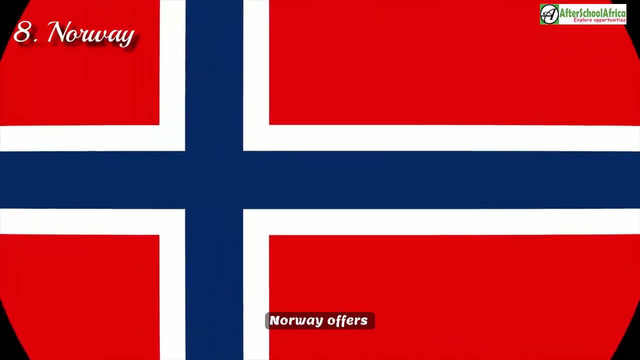 With a literacy rate of 99% and an unemployment rate at around 2.7%. perhaps the rest of the world can learn from the system of education in Iceland. 8. Norway: Norway offers the 8th best education system in the world, with 83.9 points. 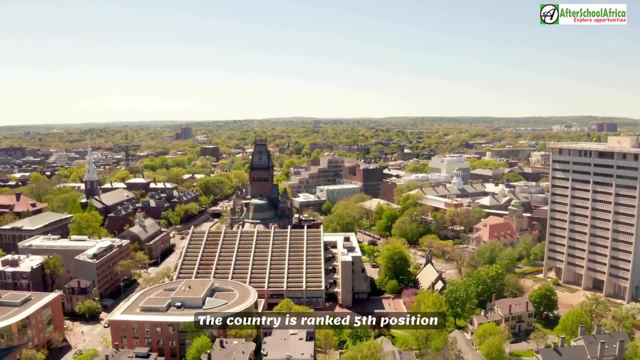 The country is ranked 5th position in school life expectancy. The country is ranked 5th position in school life expectancy. The country is ranked 5th position in school life expectancy. The country is ranked 6th position on Ease of finding skilled employees: 4th position. 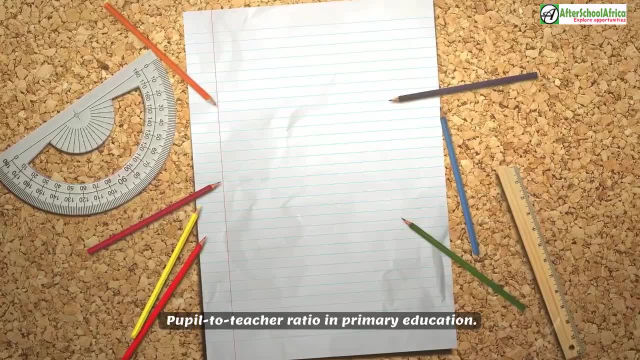 on popular cities, and 4th position on呎agnimendという ue´nust established school EL-pc policy: Functional tests on the calculations of who´s most likely uneducated population being the minority population. The Norwegian educational system is based on the principle that everyone should be able. 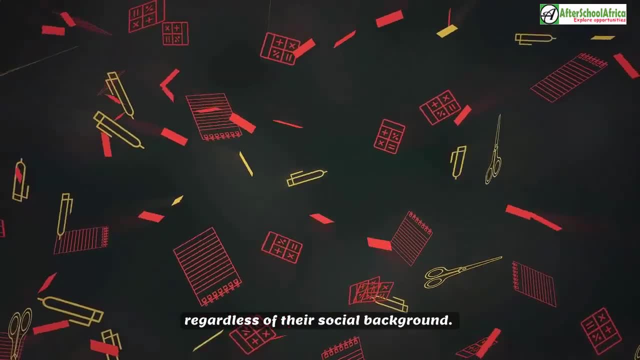 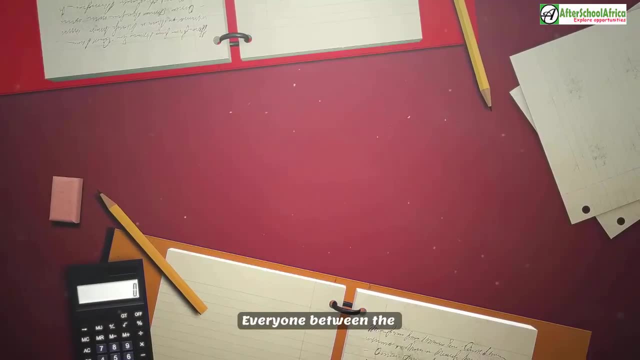 to get an education regardless of their social background. Changing standards question. The public educational system is one of the best and most popular in Europe. Thank you for listening to our decade watch up to number 5 pointest: everyone between each age from 6 to 16 must attend school in Norway. 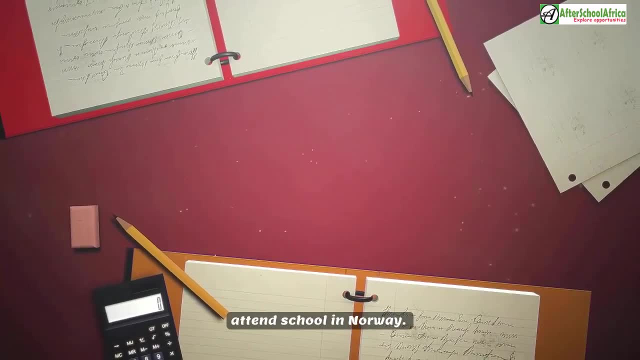 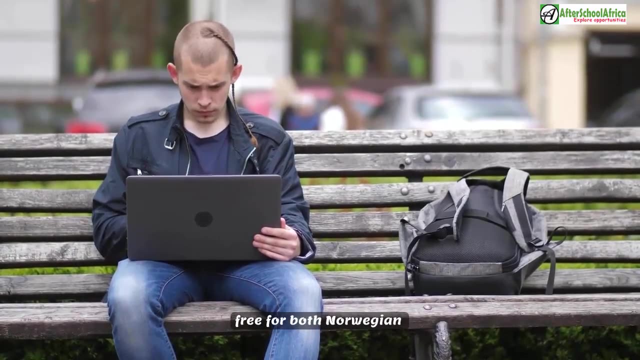 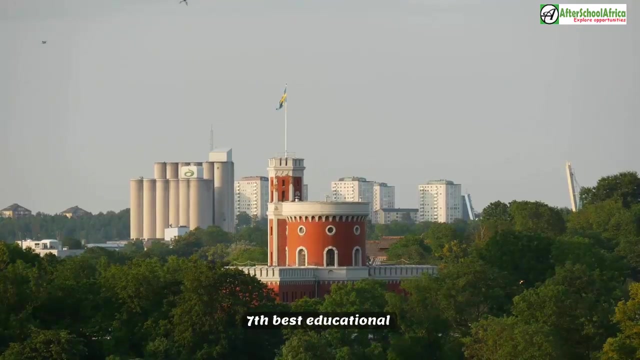 The werdke alliance, sunbae japanese institutionsreaming universities. salvation iyi, Let´s All. public education is free in Norway and public high education is tuition free for both Norwegian and international students. number seven: Sweden. Sweden offers the seventh best educational system in the world with. 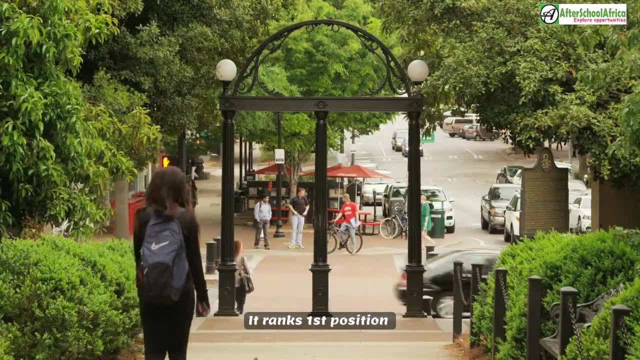 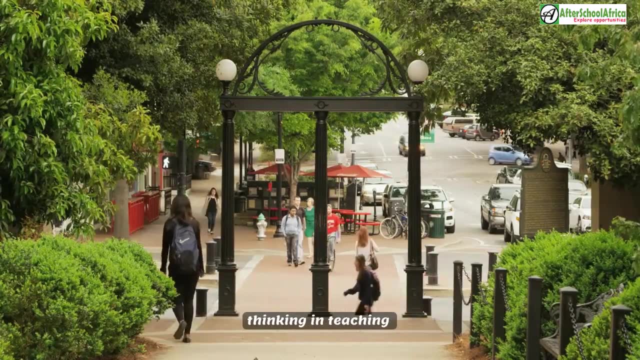 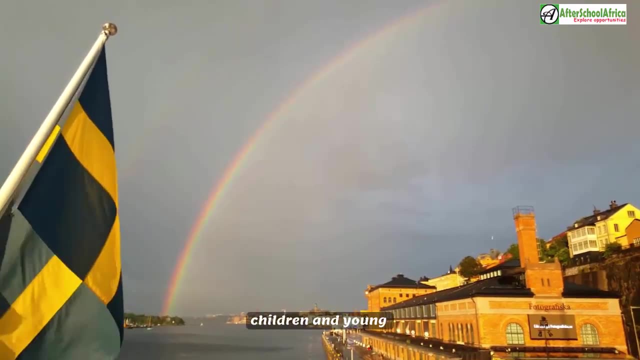 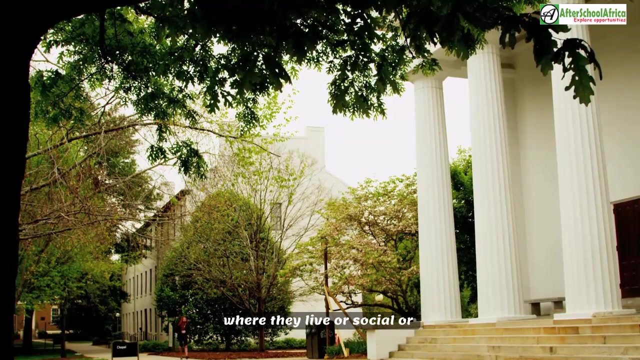 84 points. two points its ranks: first position for digital skills among population, six for critical thinking in teaching and seventh for extent of staff training. the Swedish Education Act States that all children and young people are to have equal access to education, regardless of gender, where they live or social or economic factors. 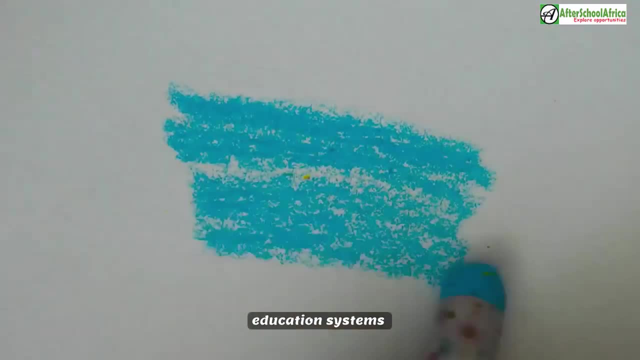 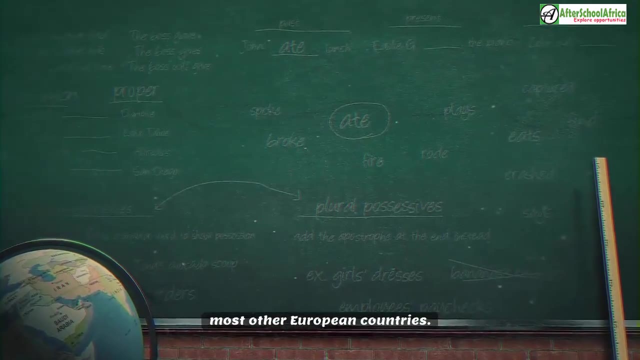 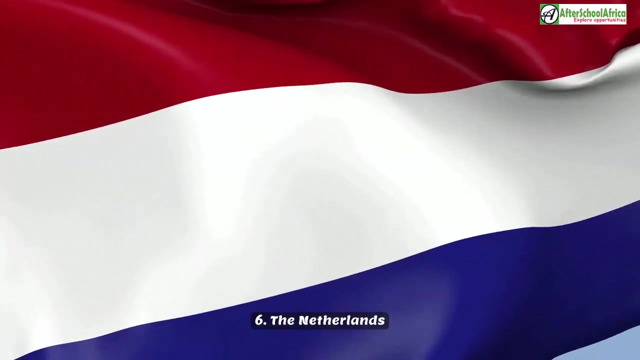 Sweden has one of the most egalitarian education systems, with pupils chances of succeeding in school Being more equal in Sweden Than most other European countries. the whole system is less target-driven and more child-centered. number six: the Netherlands. the Netherlands ranked sixth position for country with the best education system. 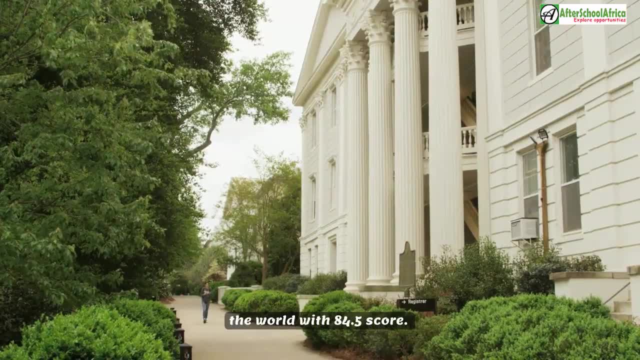 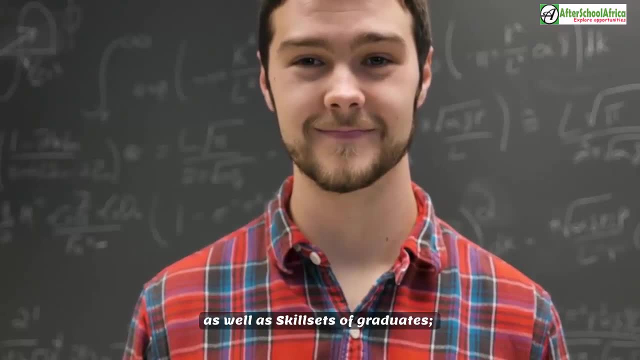 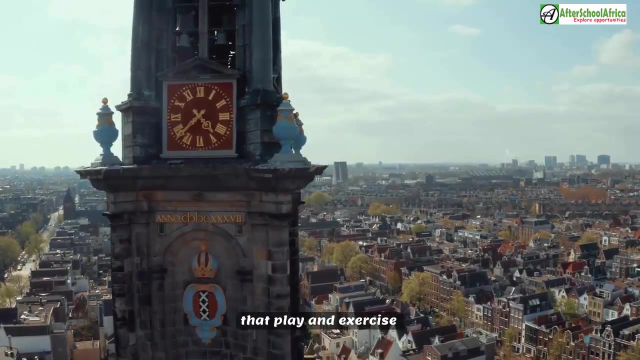 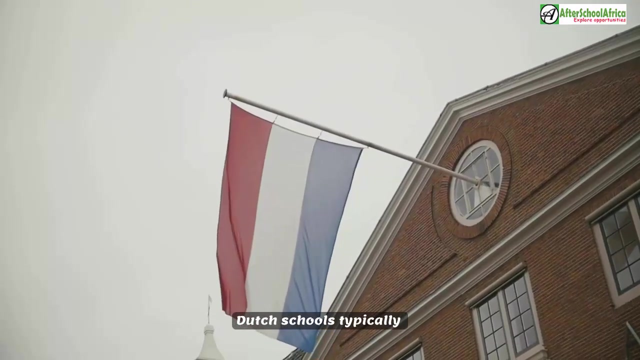 in the world with 84.5 score. it ranks third place on quality of vocational training as well as skill set of graduates, and fought on digital skills among population. Research has shown that play and exercise are vital to children's growth and school performance. Dutch schools typically don't give much homework until secondary level. 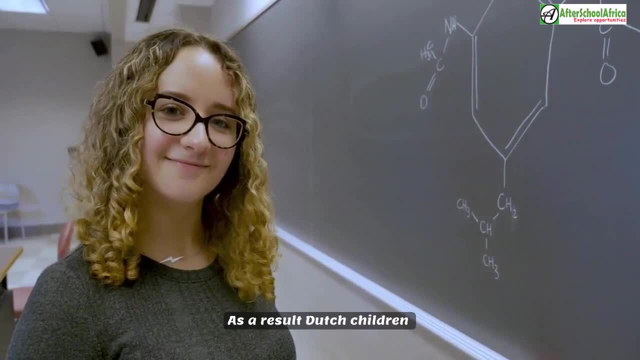 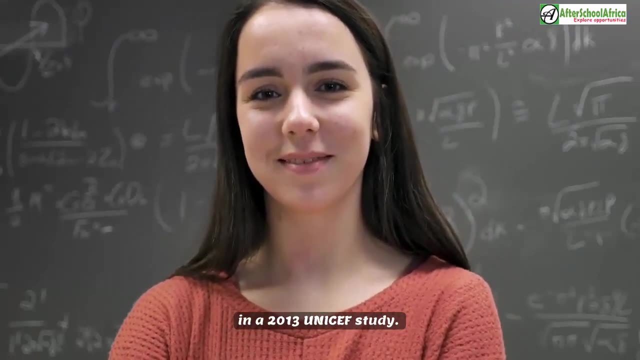 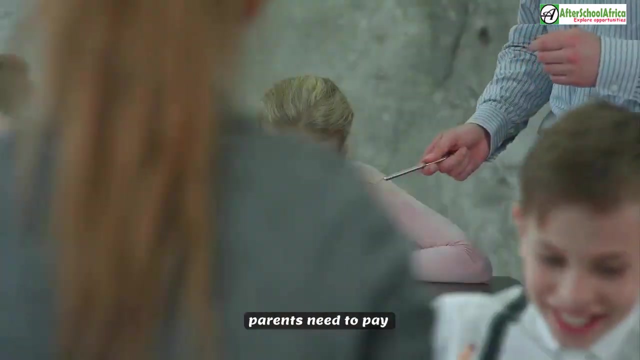 Which gives them time for daily exercise. as a result, Dutch children Were found to be the happiest in the world in a 2013 unicef study. education in the Netherlands is free for primary and secondary schools. parents need to pay for for annual tuition only after their child reaches 16 years of age. number 5: 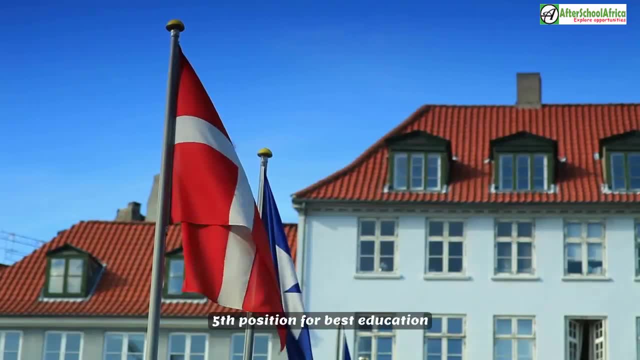 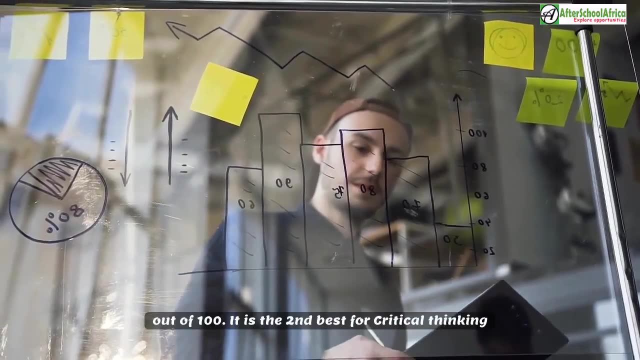 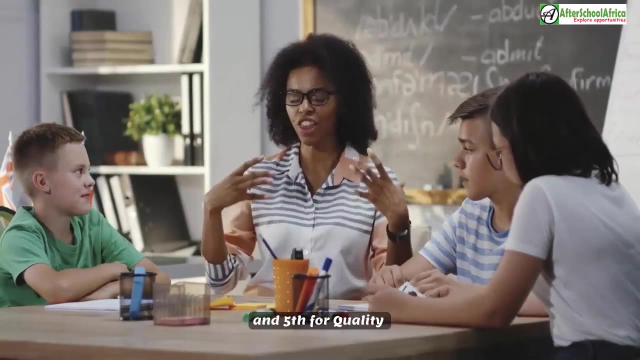 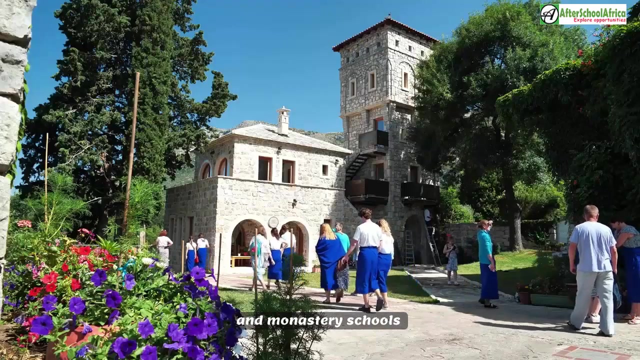 Denmark. Denmark ranks fifth position for best education system in the world with eighty four point nine points out of 100. it is the second best for critical thinking in teaching and fifth for quality of vocational training. the Danish education system has its origin in the Cathedral and monastery schools. 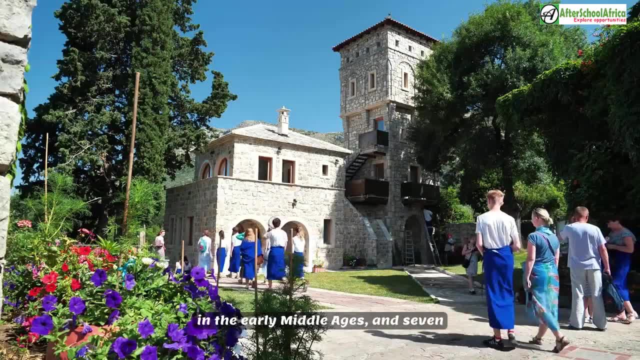 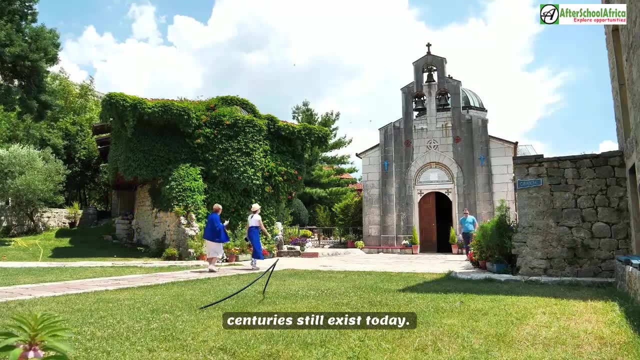 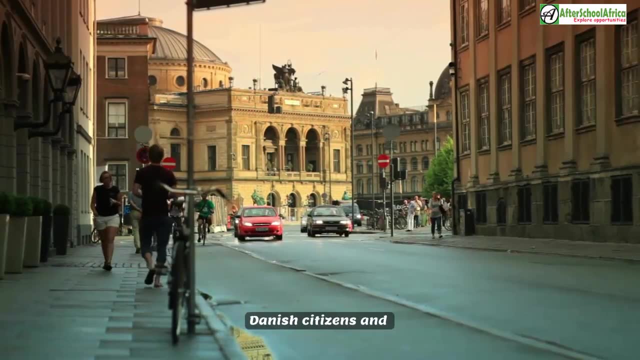 established by the Roman Catholic Church in the early Middle Ages, and seven of the schools established in the 12th and 13th centuries still exists today. almost all educational institutes in Denmark are free of charge for Danish citizens and permanent residents. education in Denmark is compulsory for children below. 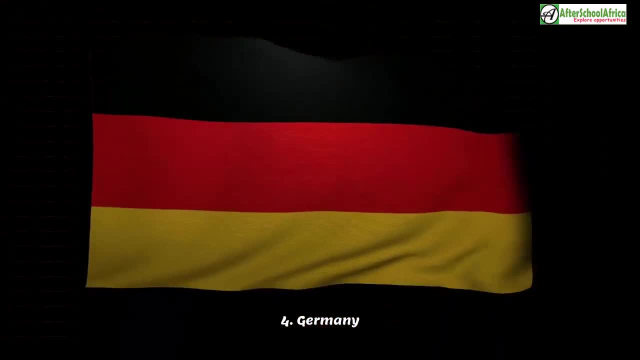 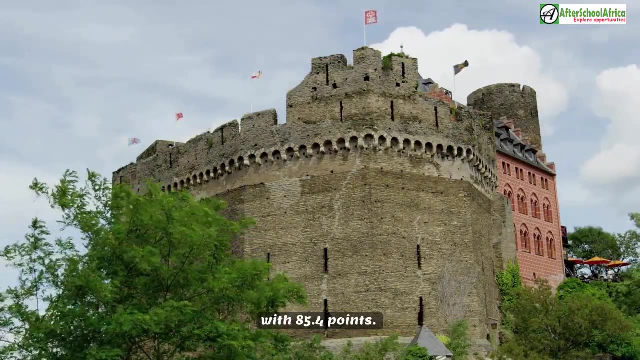 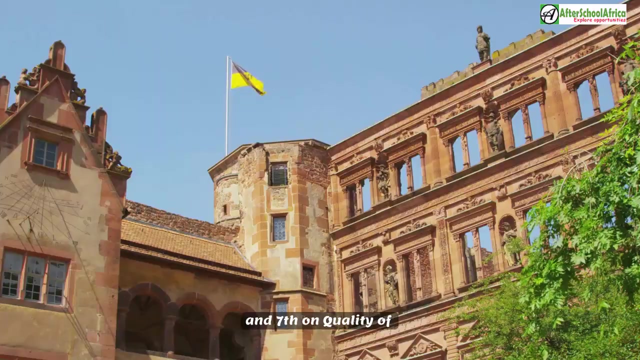 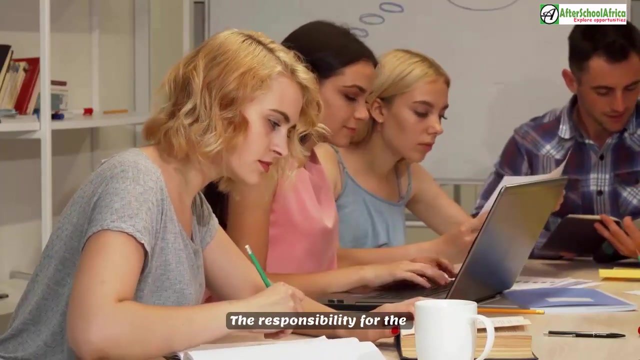 the age of 15 or 16. number four: Germany. Germany ranks fourth position for the best education system with eighty five point four points. it ranks second on mean years of schooling and seventh on quality of vocational training, skill set of graduates and ease of finding skilled employees. the responsibility for the 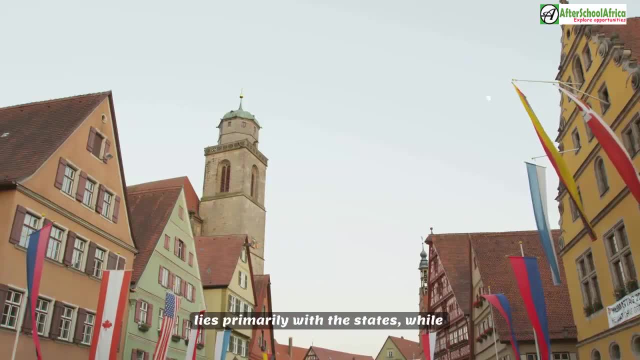 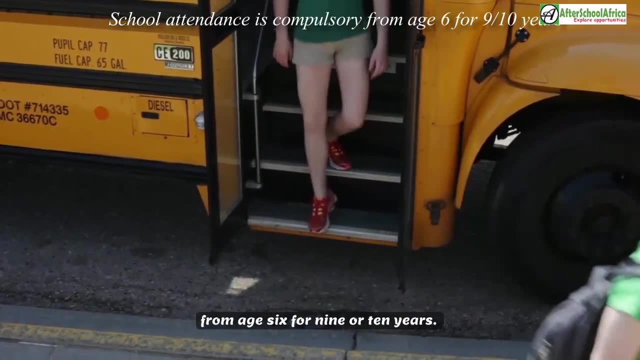 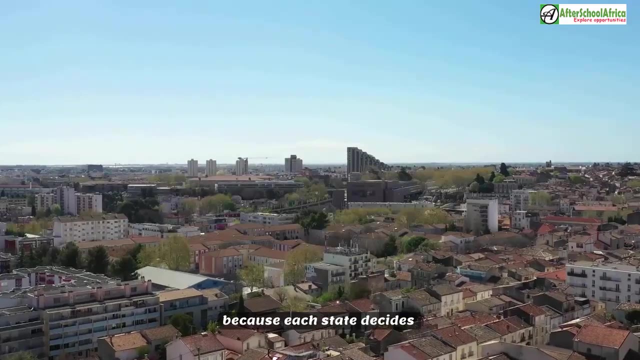 education system in Germany lies primarily with the states, while the federal government is responsible for the education system in Germany, and the federal government plays a minor role. school attendance is compulsory from age six, for nine or ten years. the system varies throughout Germany because each State decides its own educational policies. 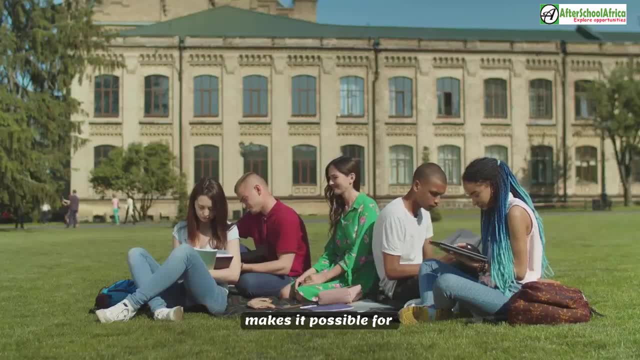 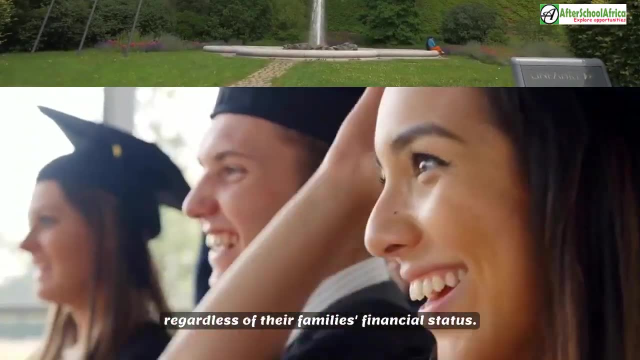 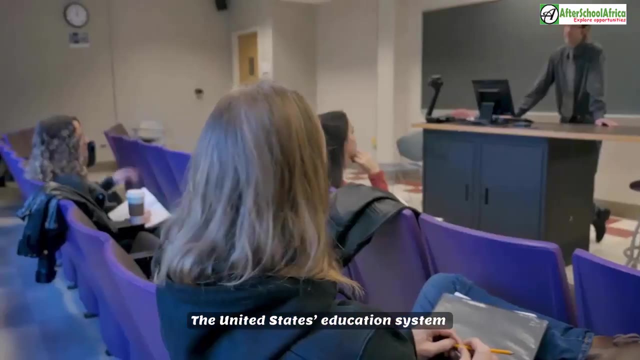 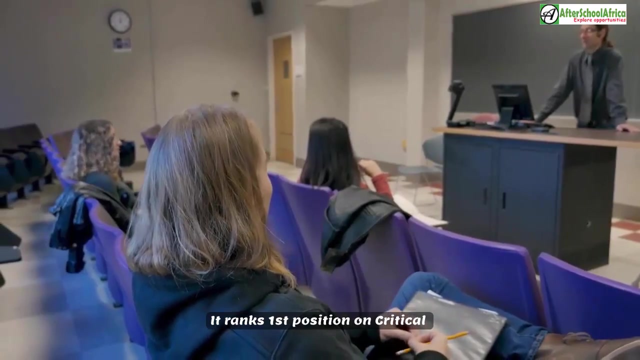 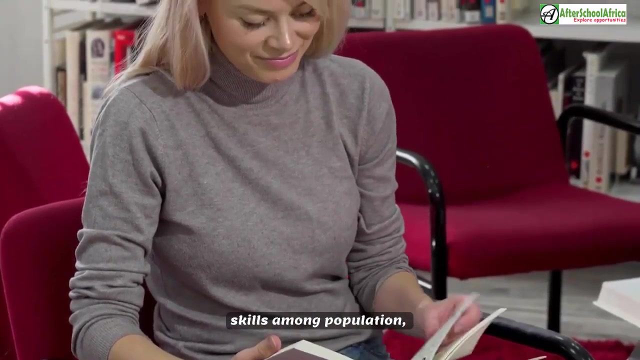 German public education makes it possible for qualified kids to study up to university level regardless of their families, financial status and United States. the United States education system ranks the third best in the world. its ranks: first position on critical thinking in teaching and ease of finding skilled employees. second position on digital skills among 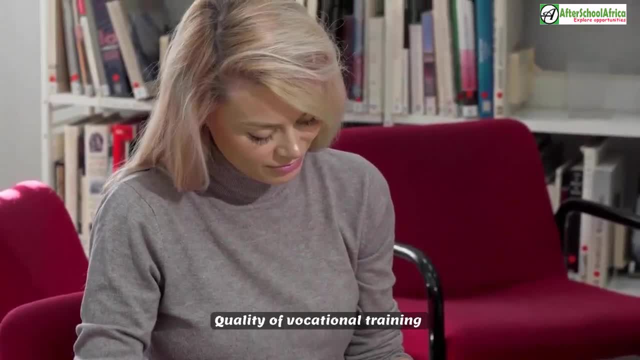 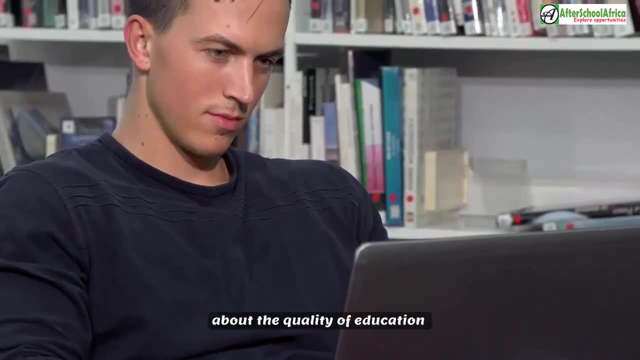 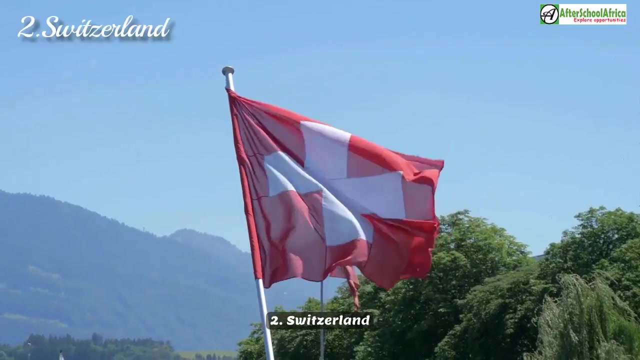 population, skill set of graduates, quality of vocational training and extent of staff training. while they are mixed debates about the quality of education in the United States, it still stands as one of the best in the world- number two: Switzerland. Switzerland has the second best education systems in the. 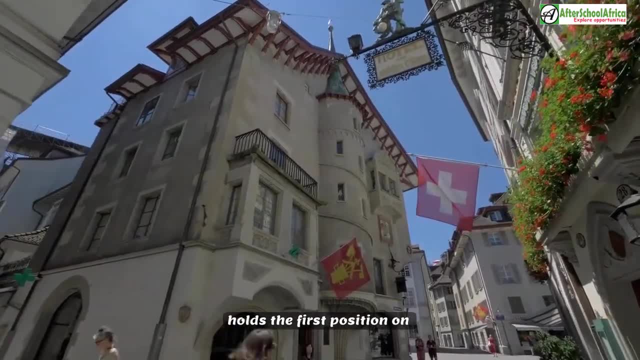 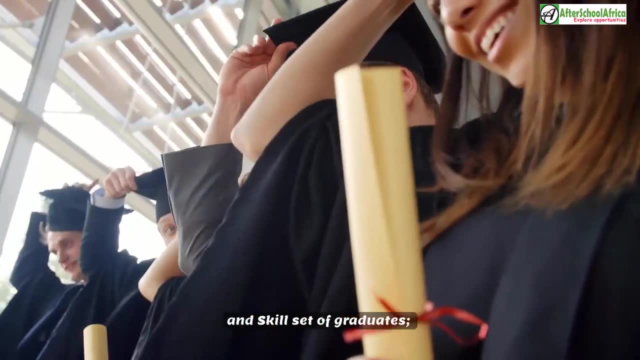 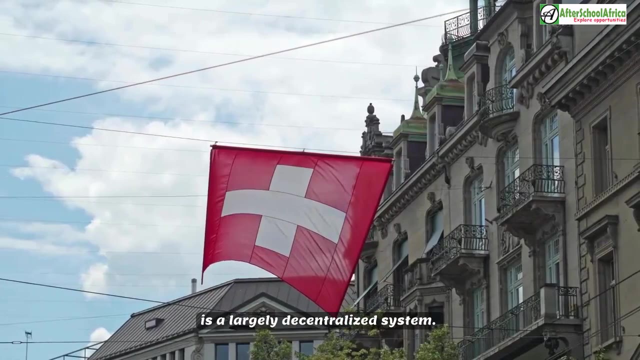 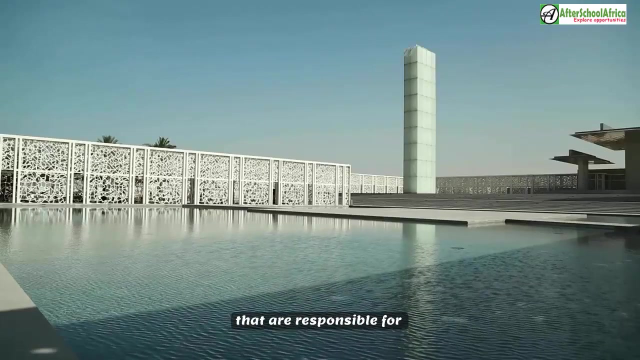 world. it holds the first position on extent of staff training, quality of vocational training and skill set of graduates, and third on critical thinking in teaching. education in Switzerland is a largely decentralized system. it's the 26 cantons, not the federal government, that are responsible for their compulsory education system, and the system relies almost entirely on 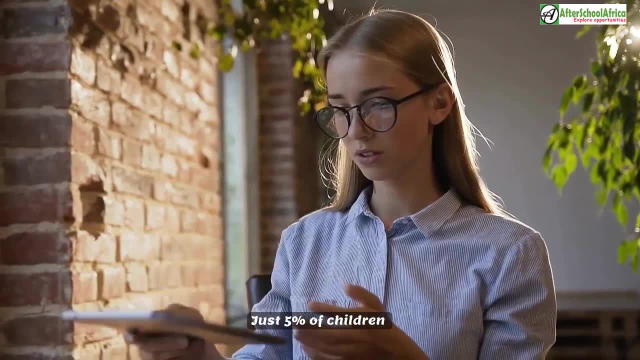 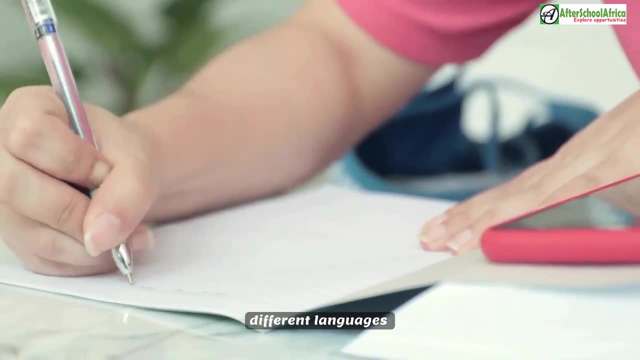 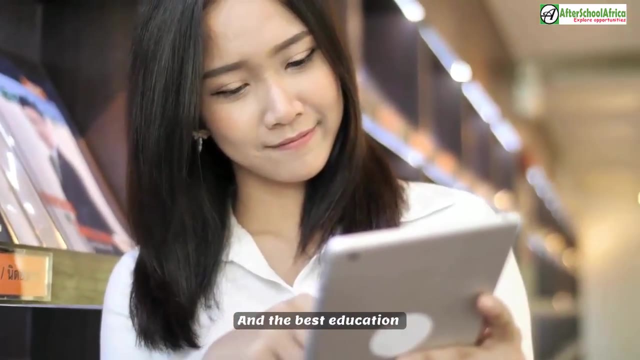 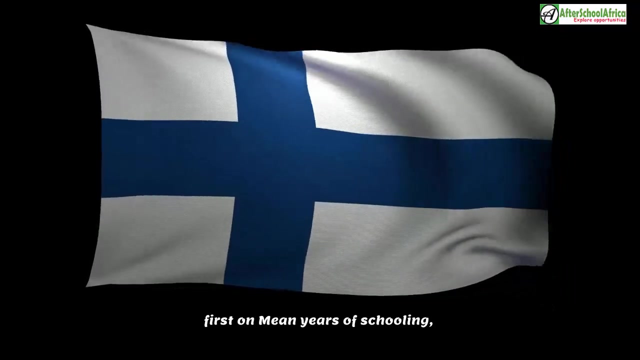 public fund. just 5% of children attend private schools, the rest go to public schools. lessons are taught in different languages, including Germany, French and Italian, depending on the region of Switzerland, and the best education system in the world is found in Finland. Finland ranks first on mean years of.